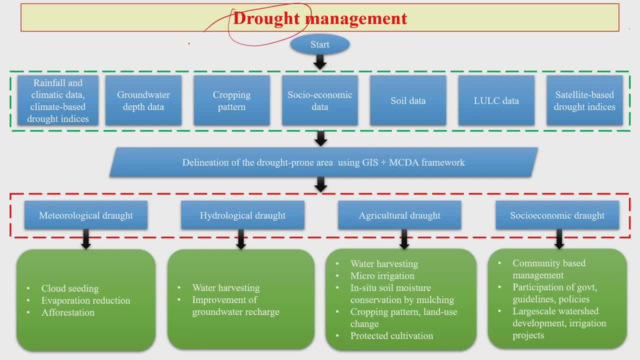 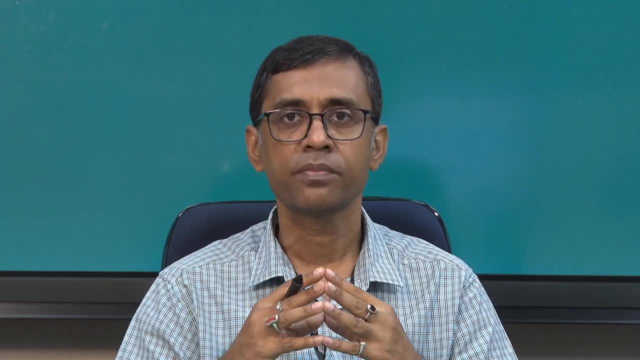 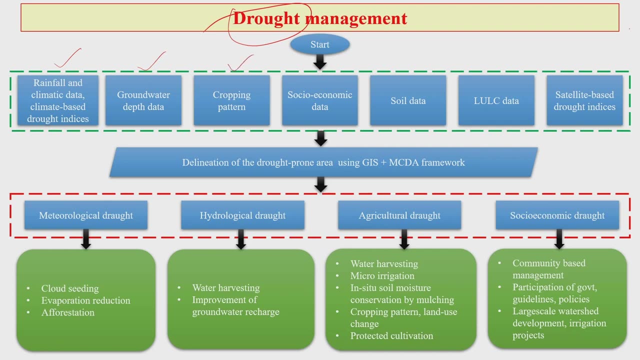 within a watershed, and that is about drought. Now, like flood, the drought management also depends quite significantly on the data that actually you have with you. So the drought management system: it is based on your rainfall data, climatic data, climate based- different. 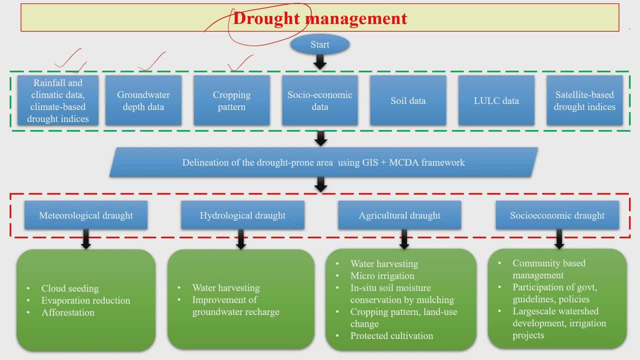 drought indices, ground water depth data, cropping pattern, socio-economic data and soil data very important household level information, soil data, land use, land classification data, satellite based drought indices. So these sets of data, when you have with you, 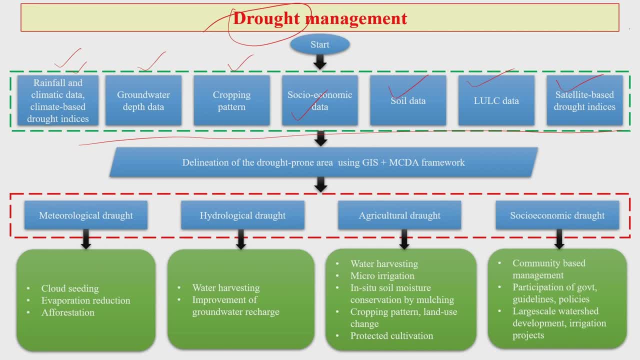 you actually have treasure in your hand Now. on the basis of these databases or data, you start actually delineating of the drought prone area using tools like geographic information system, multiple criteria, decision making system and so on. So this can be carried out independently through GIS and MCDA, but you can also bring these 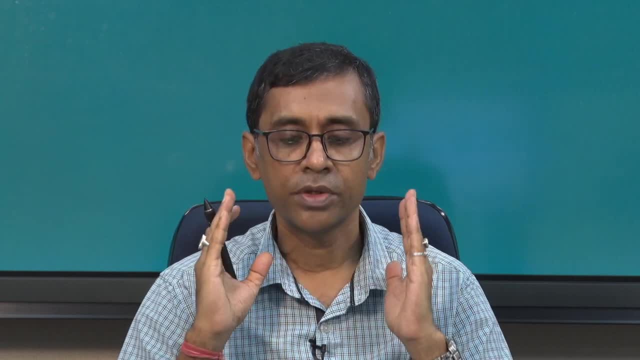 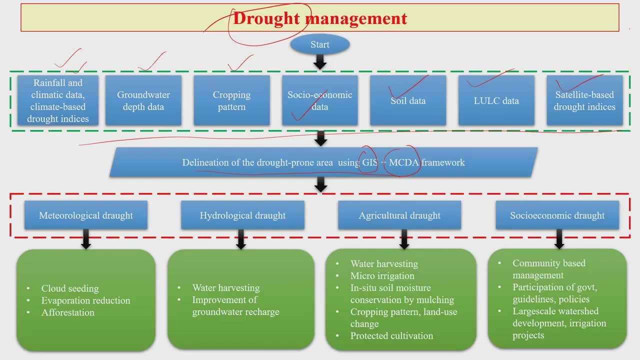 two powerful tools together for better decision on the basis of your alternatives that are available for drought management. Now let us see that: what different kind of droughts that you can actually expect, because on the basis of the type of the drought, we need to decide on the management. 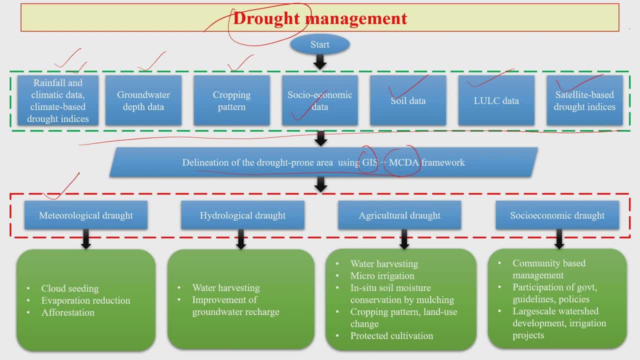 Let us see how well the management practices. Now, meteorological drought. we have hydrological drought, agricultural drought, socio-economic drought. now, each one of them from the name itself, you can very well understand that they have a different manifestation of single phenomenon that is drought. So certainly meteorological. 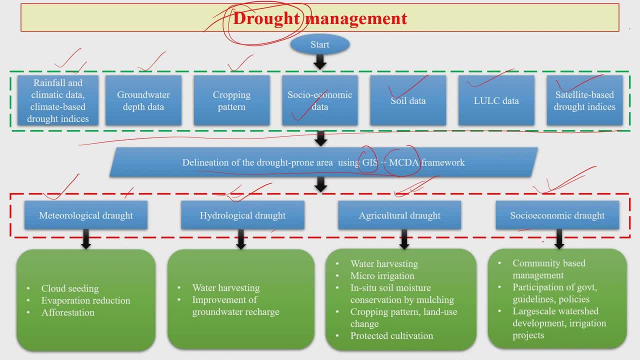 drought, hydrological, agricultural, socio-economic needs, different type of management practices. let us see how, actually, we could actually approach each one of them. the metallurgical drought means the drought which is largely depending on the metallurgical parameters. so what are the options? 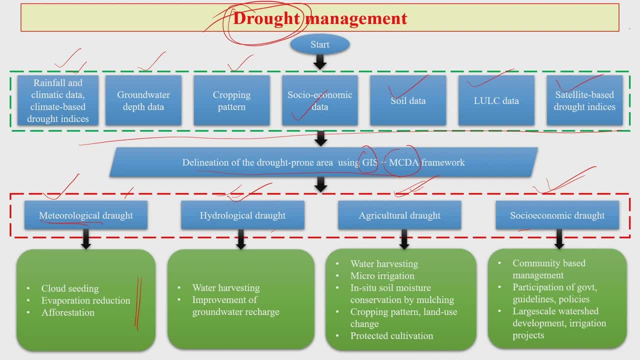 or management practices that actually you can try for managing metallurgical drought clouds- seeding, evaporation reduction, afforestation- easiest but very, very efficient hydrological drought. in hydrological drought you will see that the previous discussion that we had on watershed management, so from there in fact we can also find out the different approaches. 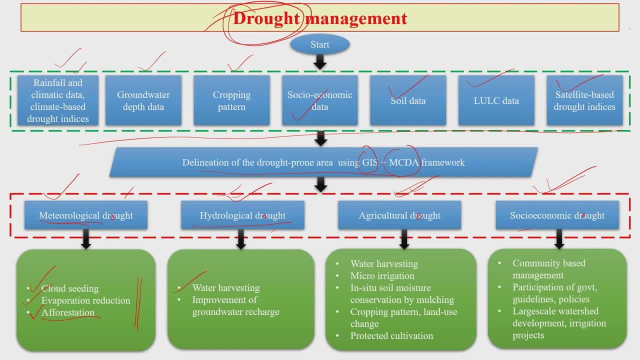 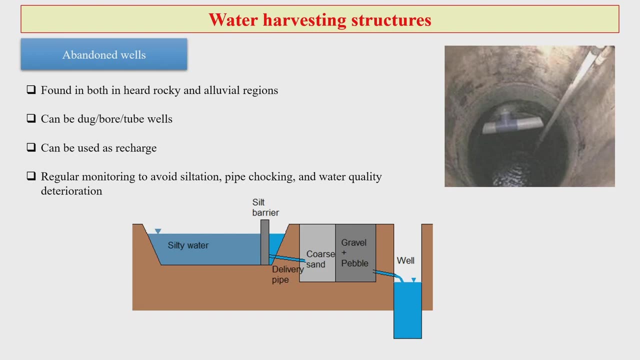 for addressing hydrological drought. so water harvesting- already we discussed that, how we can do that. improvement of groundwater recharge also we have discussed in the previous slides. we have discussed in quite detail that what are the different kind of water harvesting we could do, and also various other. 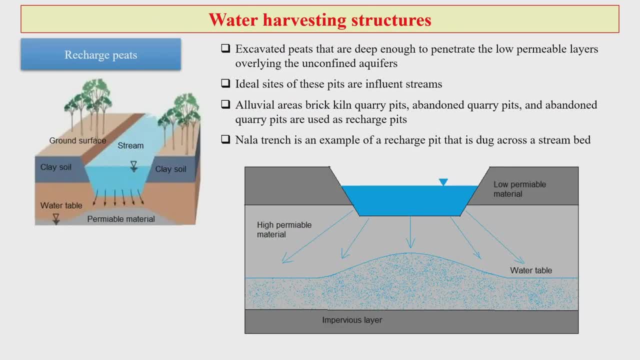 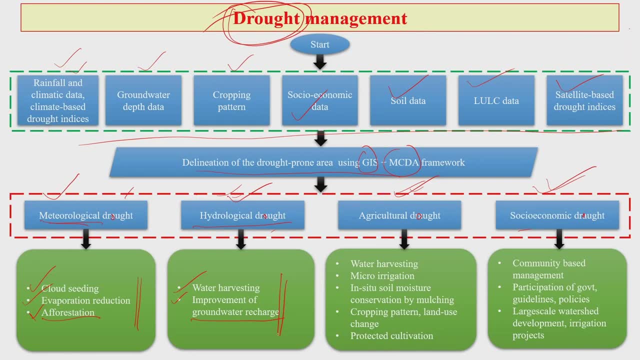 approaches for land use management and water management. so once you have also this kind of techniques with you, you can actually try them for any watershed, for hydrological drought management, agricultural drought- it is bit complicated in comparison to the other two, so in case of agricultural drought, here you are actually going to, you know, deal with water. 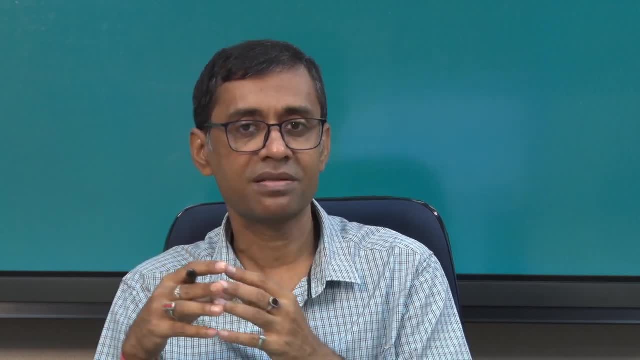 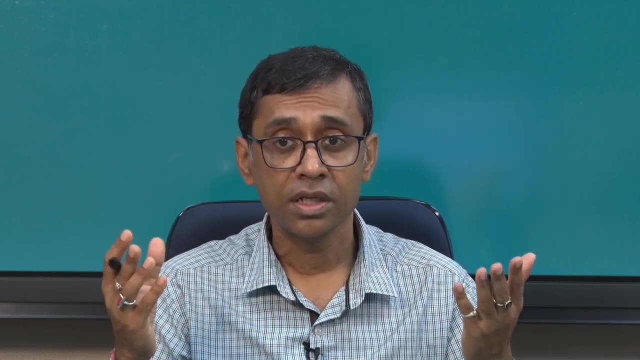 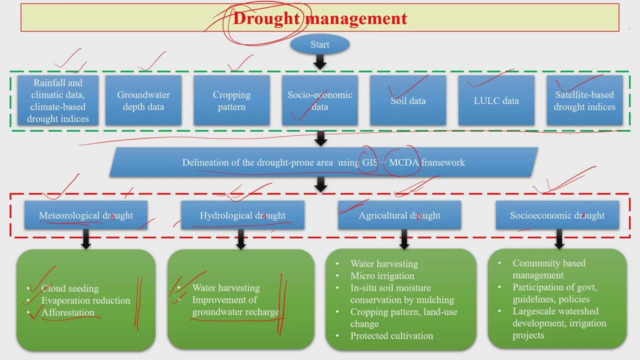 importance of water and impact of water scarcity on productivity, which is directly connected with the livelihood of the people and also their sustainable well-being. so here again some of the practices that we tried. you know, for the other two kind of drought, water harvesting is actually a kind of a magic key for most of the problem that you have which are related to water. 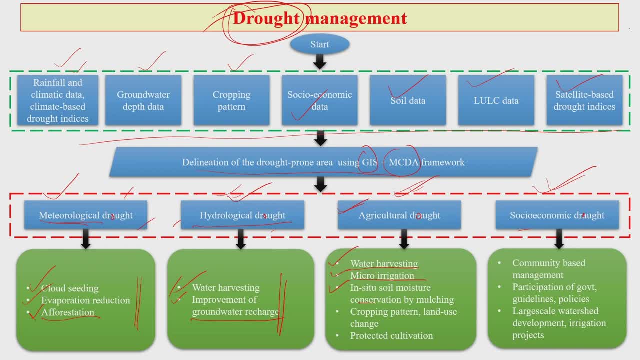 for, in case of watershed, micro irrigation, in situ soil moisture conservation by mulching that could be leaf litter munching, and we also discussed about, you know, plastic mulching, which a那 personally do not recommend in every cases. but if you are have large kind of you know farm, then definitely plastic munching can be of good use. otherwise i think that we have huge growth. other depends the situation and of course, for that i think it is very important that we still try to correct the problems of the previous side. that's why i am saying, in terms of the development, we guys 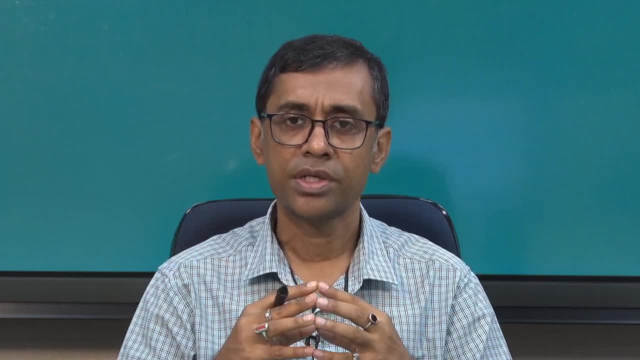 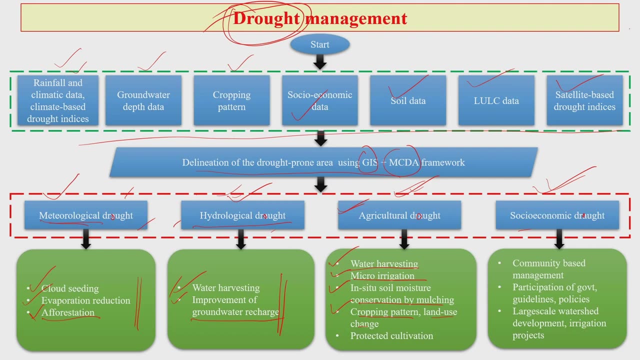 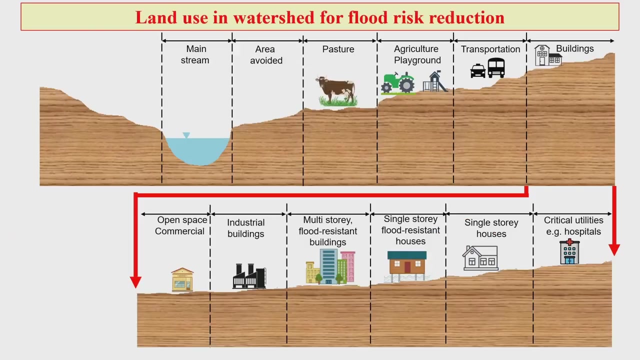 어제 sa y. I think that we should go with our indigenous material like leaf litters and etcetera for in-situ soil, moisture, Cropping pattern and land use change. again I think we have, if you recall that we have discussed all those things in quite detail about land use for various purposes. 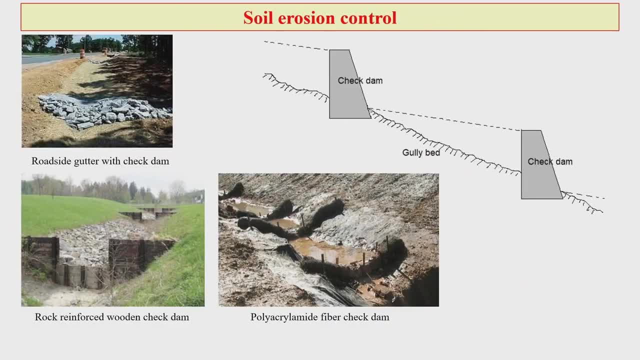 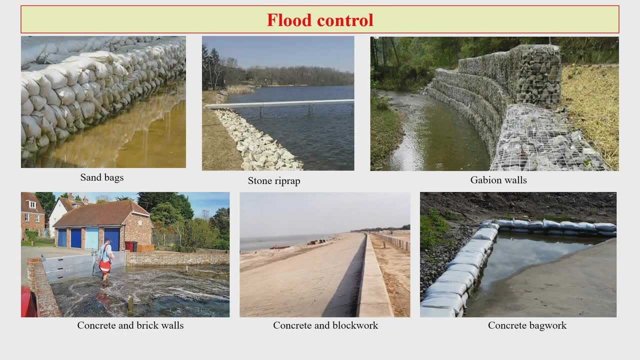 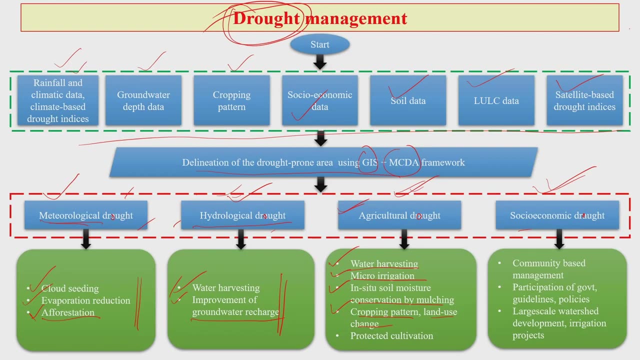 We also discussed about the groundwater recharge and erosion control. So I think that you know the previous lectures are very important that you refer to when we talk about drought management. So agriculture, drought management also critical for another reason. that is because you are actually going to, you know, lose your crops if you are not able to give the water at the 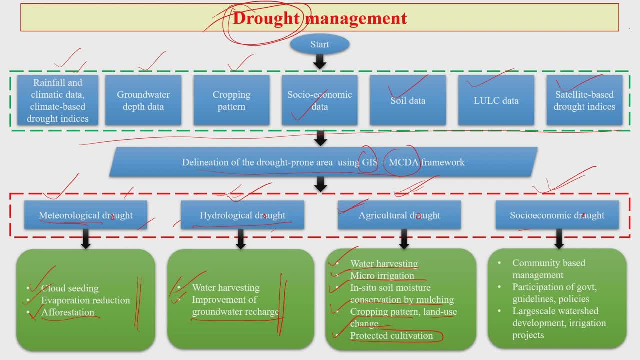 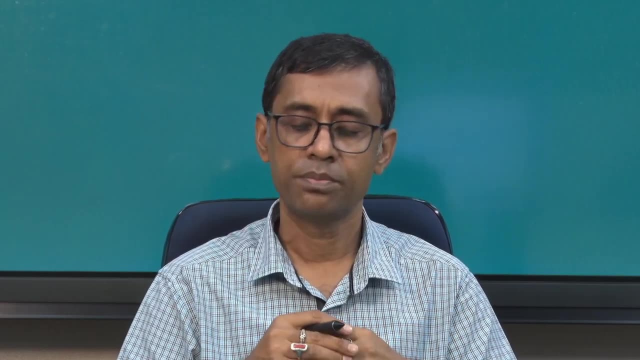 right moment, alright. So protected culture Cultivation is another very new type of cultivation practices which in many places, of course in the developed country, are being utilized, but in India also, many places this protected cultivation are being used for, you know, addressing the agricultural drought. 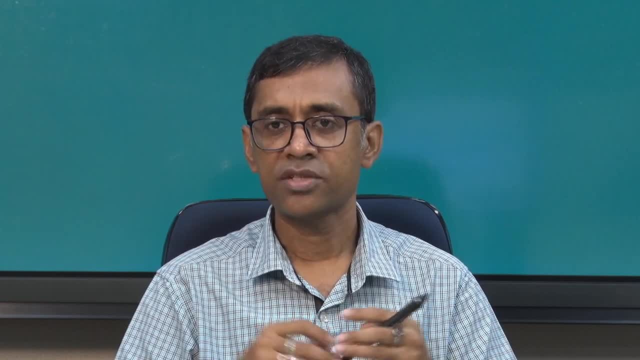 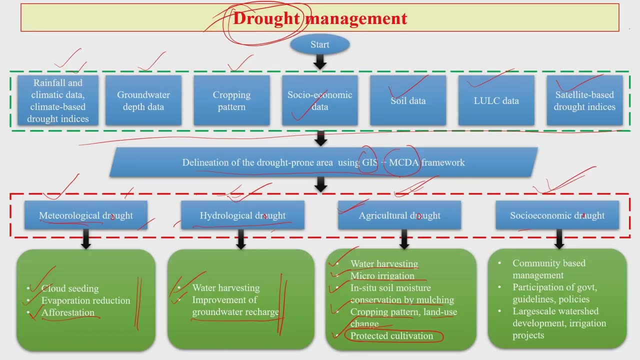 So when you say protected cultivation, that means it is actually to protect your cropping system for any kind of adversity. In this particular case, it is drought, Socio-economic drought. again, it is very important from the perspective of the community and the people, because everything that we have been discussing is actually related to. ultimately, 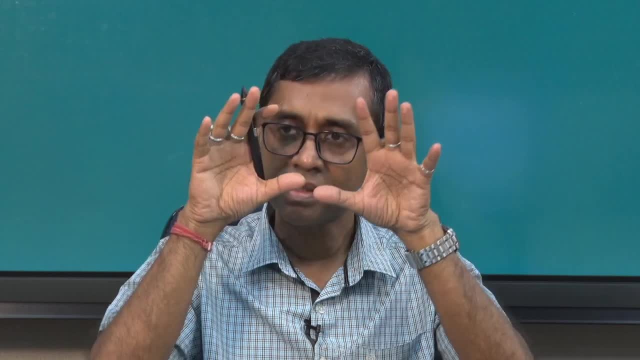 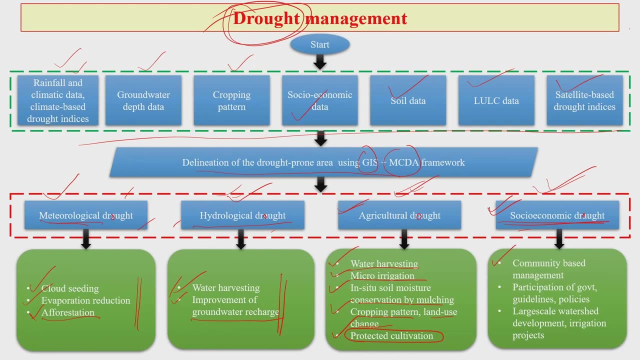 to human. So the society is right at the center of our discussion, right. So socio-economic drought actually is important from that point of view. anytime when drought takes place or flood takes place, Any natural disaster, Any natural calamity, Immediately the first effect is that the livelihood gets somehow disturbed. 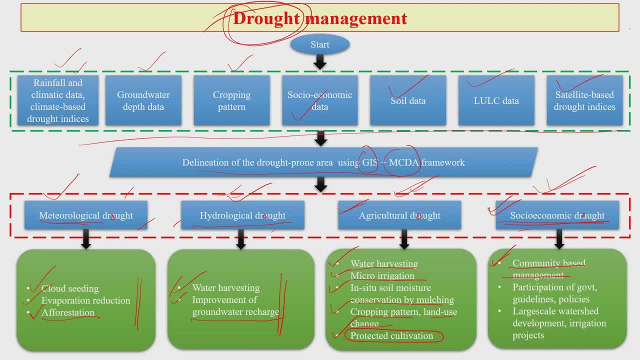 So community based management is one way that we can address socio-economic drought. participation of government following guidelines policy, large scale water development, irrigation projects are some of the tools and techniques that can be used for addressing socio-economic drought. So as you see overall that in case of flood as well as drought management, we need a mix, 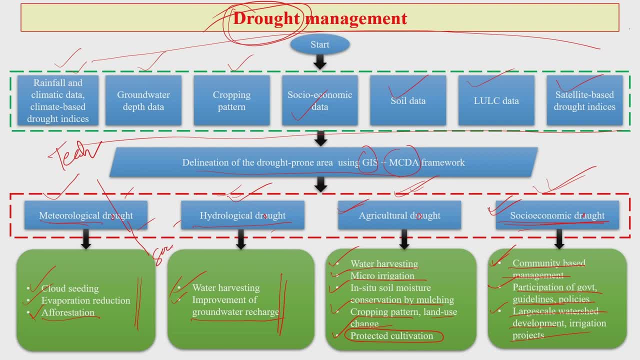 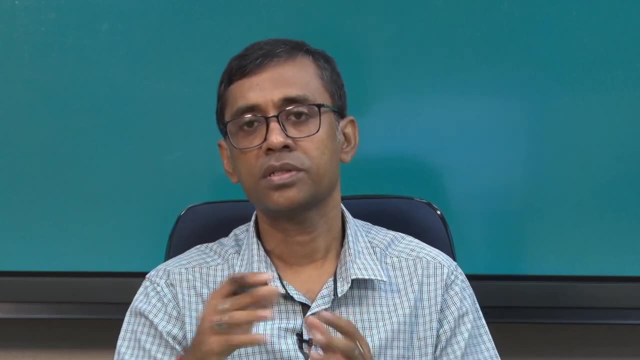 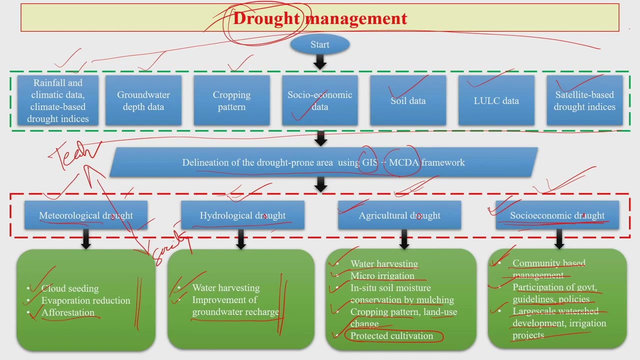 of technology and society. So a perfect combination of technology and society will definitely lead to sustainable management of your watershed and thus also ensure the sustainable well-being of the community. Next, In case of, especially the cloud seeding that we just now discussed about: meteorological 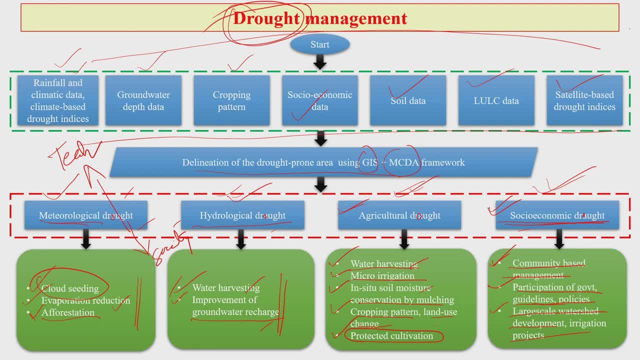 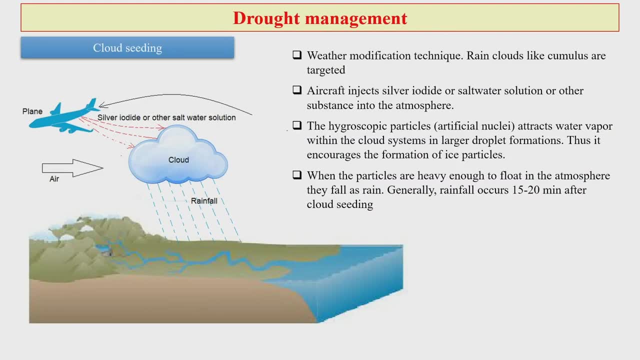 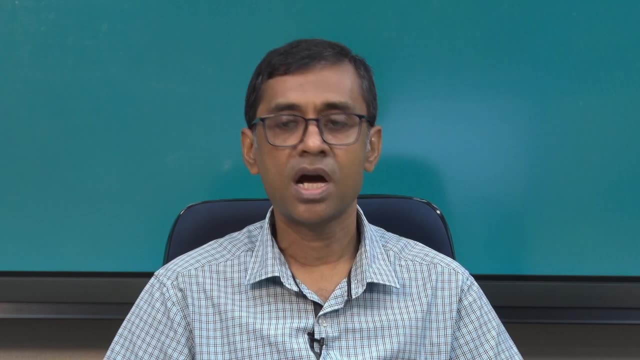 drought because rest of the things I am sure that most of you are well aware of and many places these are being followed also. I just would like to take the case of cloud seeding, because that has become a kind of a very popular way of managing drought, mostly in the developed. 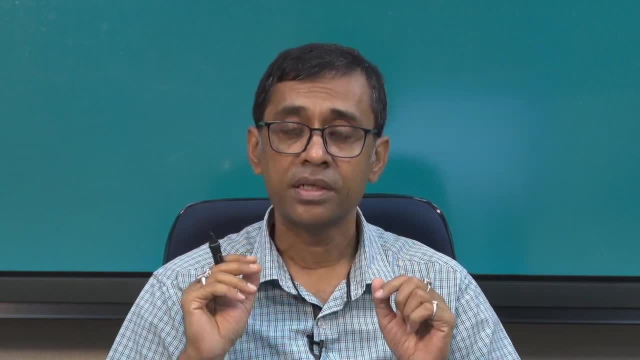 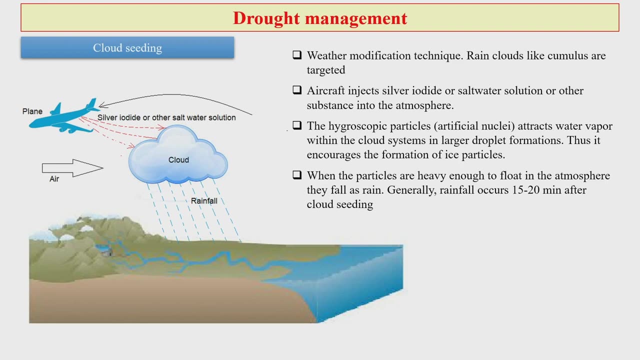 countries, But we can also try In India, So why not? to see that how these actually work? So in case of cloud seeding, basically you know a plane is being used and what you actually carry, in that you carry silver iodide or other salt water solution which you basically sprinkle. 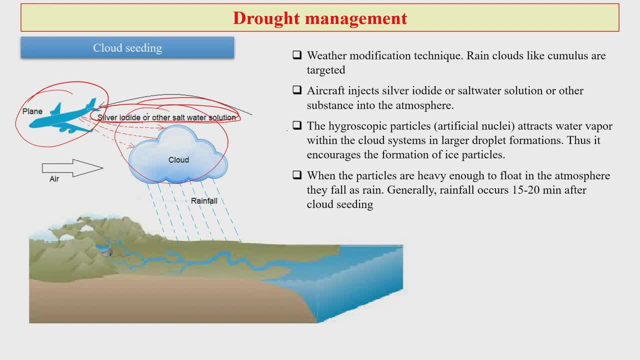 or spray into the environment, in which actually form a kind of a cloud, basically, And then Next, In presence of low temperature and movement of air, finally that cloud, will you know, convert it into rainfall and then you get the water. So weather mode, it is a kind of a weather modification technique, and rain clouds, like 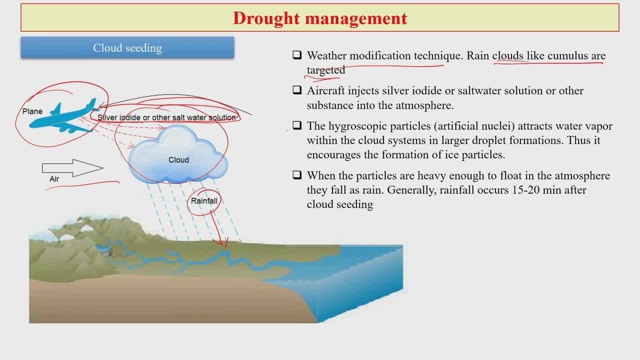 cumulus are largely targeted for that. What aircraft actually? your plane? does aircraft inject silver iodide or salt water solution or others substance, as I said, into that model? So what is the it into the atmosphere and these hygroscopic particles which actually being sprayed or 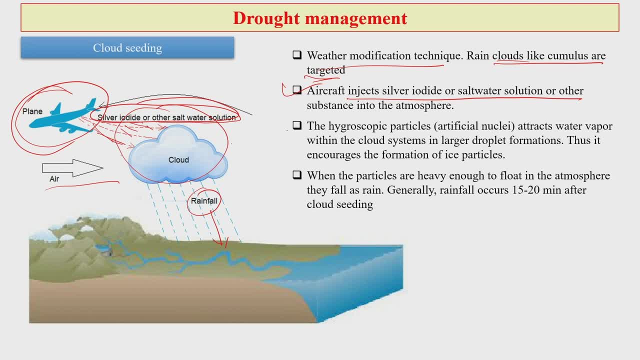 sprinkled from the aircraft. it attracts water vapour from the ambient environment within the cloud system in larger droplet formation. what is actually it does is that it forms larger droplet within this particular, you know, cloud, which has been formed already there, So thus it encourages the formation of ice particle. 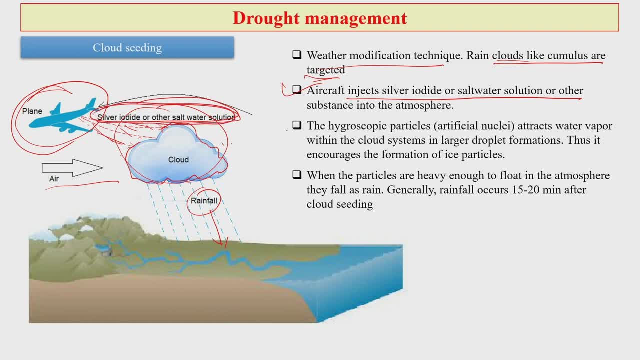 So the large droplet, first of all silver iodide. this comes into the cloud, helps the small water droplet to become, you know, a bigger droplet. then, under the low temperature and other conducive condition, it is become into ice particle, When the particles become very heavy enough, you know, and cannot float in the atmosphere. 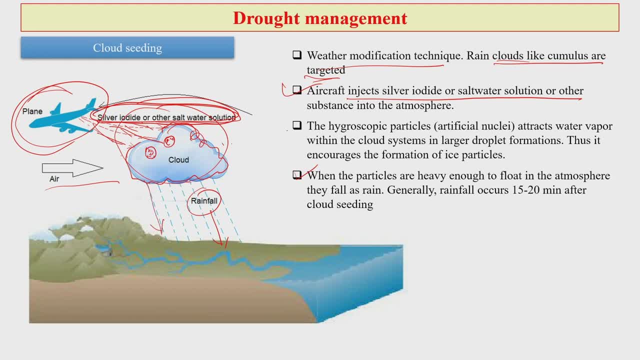 any further, Then automatically they fall, they fall, they come down to the earth. Generally, rainfall occurs, you know, 15 to 20 minutes after this kind of cloud seeding, the cloud seeding which is being done by silver iodide or other salt solution. 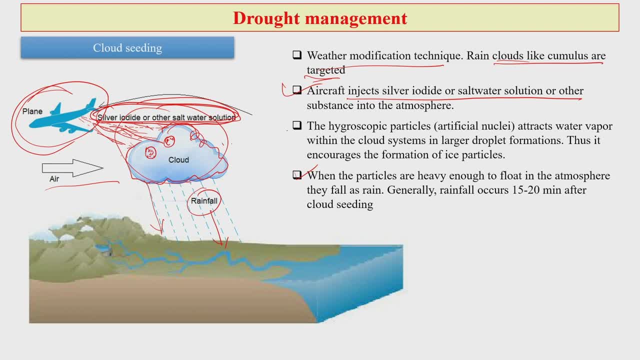 So this is one you know, artificial way of you know forming bigger droplets and forcing a rain at the time of requirement on the ground. So this is one you know, artificial way of you know forming bigger droplets and forcing a rain at the time of requirement on the ground. 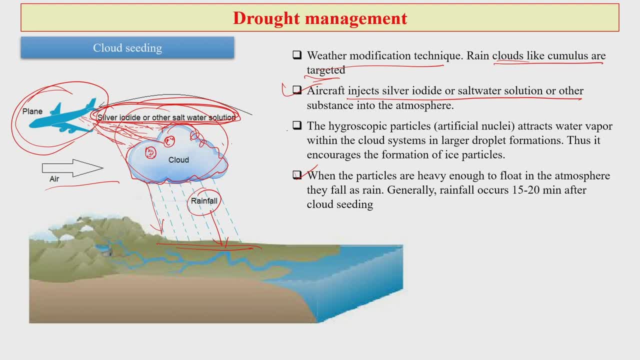 So this is one, you know, artificial way of you know, forming bigger droplets and forcing a rain at the time of requirement on the ground. I simplify this case. say, for example, in an area in Rajasthan you want to grow a crop and that crop is suppose one of the main livelihood option for that particular community. 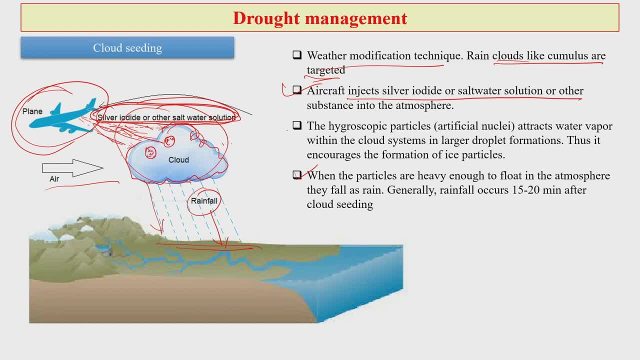 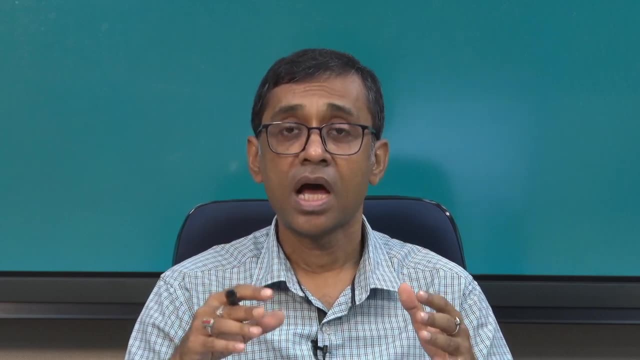 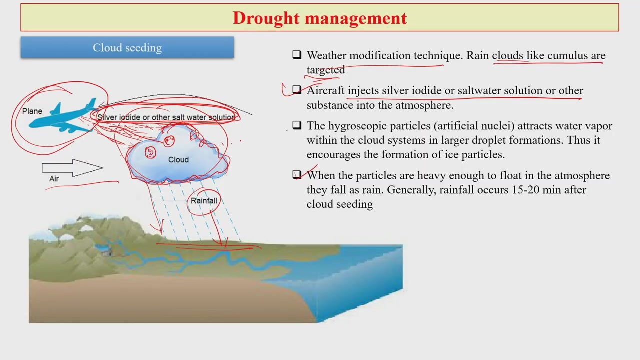 But you are sure that you are not going to get, you know, rain naturally. So how to do In that case? you probably try, you know, cloud seeding. So this basically help To bring the rain at the time when you want. Otherwise, if you leave it, this cloud to the nature completely, it might happen that never. 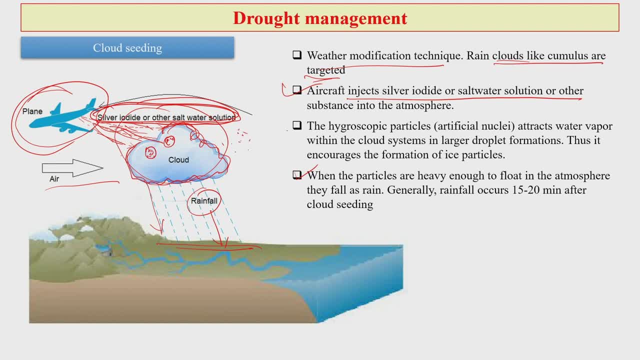 this small, tiny droplet will become of the size which finally can fall down on the earth. It can happen that the strong wind can flow away this cloud from the area where you actually want the rain. So this is how cloud seeding basically help in this case.